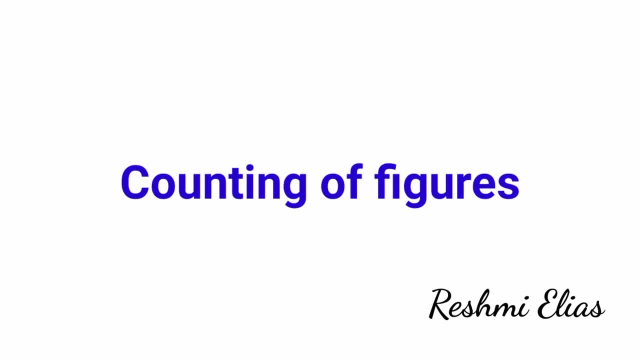 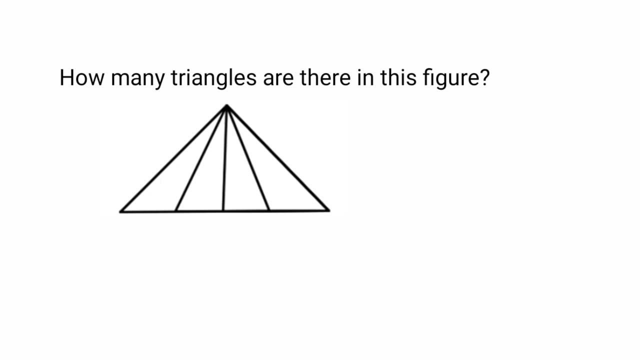 Hi all, this is Reshmi Elias from Freshersworldcom. In today's video, I will be dealing with the topic counting of figures, and this will be helpful for everyone who are preparing for various competitive exams. Our question is to find the number of triangles in this figure. Actually, it will be. 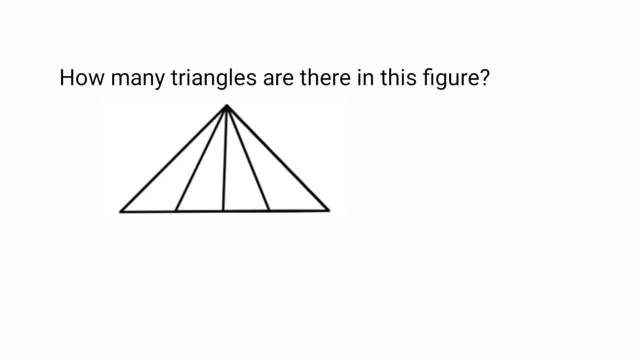 time consuming if you really want to count the number of triangles and to solve this question. So we have a shortcut for this. So what you have to do is just find the number of bases. Here there are 1,, 2,, 3, 4.. 4 bases are there, So to find the total number of triangles, 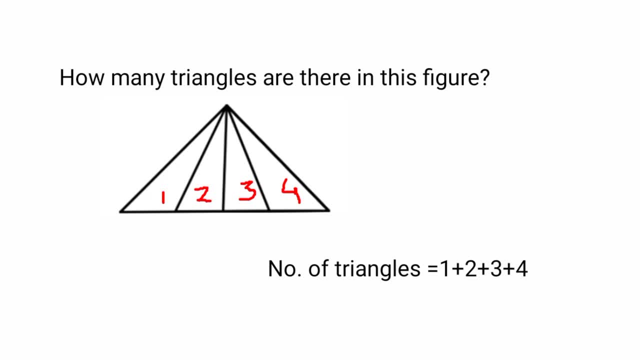 you just need to add the bases. That is 1 plus 2 plus 3 plus 4.. That is 4 plus 3 is 7, 7 plus 2 is 9,, 9 plus 1 is 10.. So the answer is 10.. So, using the same shortcut, 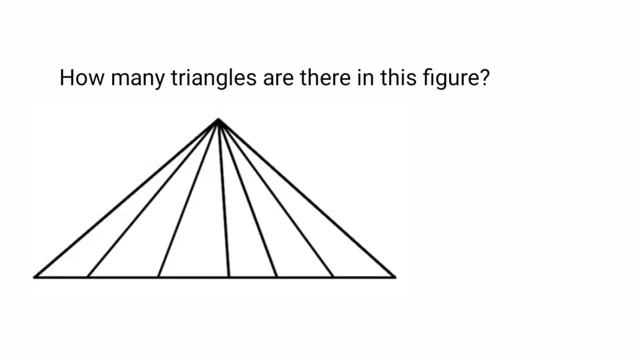 we can find out the number of triangles in this figure. So what you have to do just count the number of bases. Here there are 1, 2, 3, 4, 5, 6.. 6 bases are there. So what you have to do is: 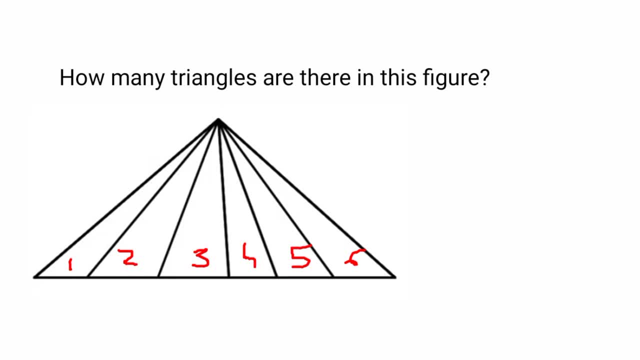 just add all these values. So 1 plus 2 is 3,, 3 plus 3 is 6,, 6 plus 4 is 10, 10 plus 5 is 15,, 15 plus 6 is 21.. But 1 plus 2, plus, etc. up to 6. This is the sum of. 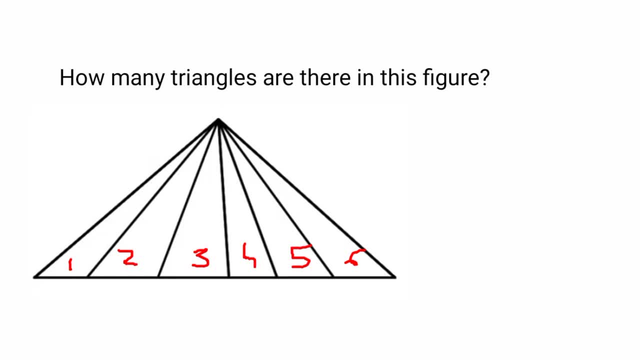 first 6 natural numbers. What is the equation for finding the sum of first n natural numbers n into n plus 1 by 2.. So here we will get the sum as 6 into 6 plus 1 is 7, 7 by 2.. We can cancel. 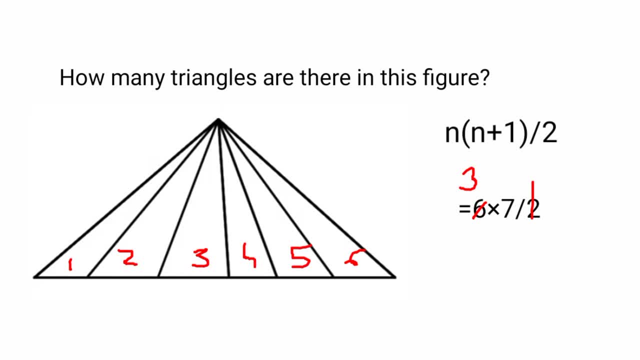 out 2 and 6, 3 times 3 into 7 is 21.. So we will get 21 as the answer. So you can use any of the two methods. That is, either you can add all these bases or you can use the equation Suppose if you want to find out the 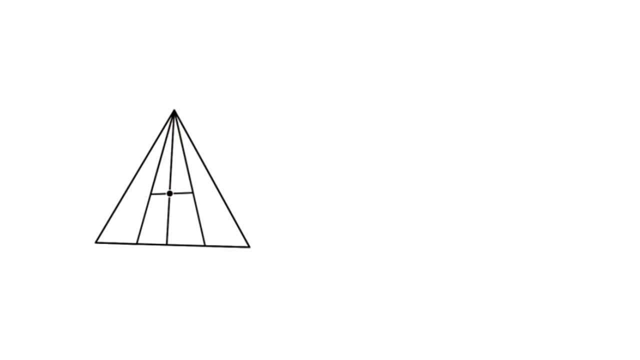 number of triangles of this triangle. what you have to do, We can follow the same steps, So count the number of bases. Consider the large triangle without division. How many bases are there? 1, 2,, 3, 4.. There are 4 bases, So how many triangles are formed there? 1 plus 2 plus 3 plus 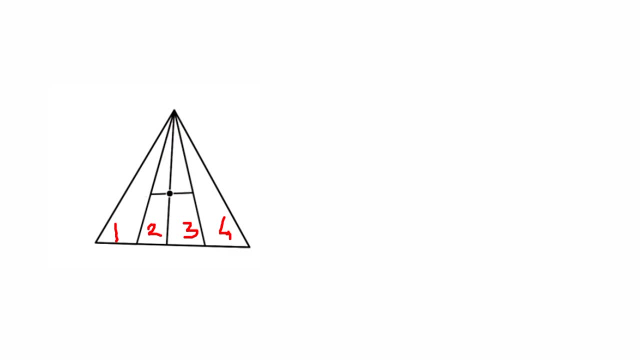 4. That is 1 plus 2, 3,, 3 plus 3, 6.. 6 plus 4, 10.. So in total, 10 triangles are there. Now consider the triangle which is formed inside. How many bases are there? 1, 2. So how many? 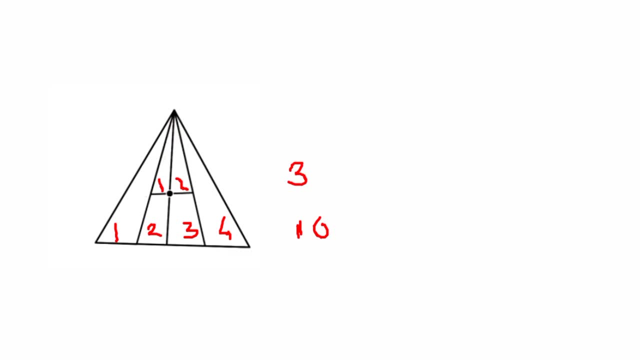 triangles will be formed there, 1 plus 2, 3 triangles, So in total 10 plus 3, 13 triangles are there. Next question is to find out the number of triangles in this type of figure. So to solve this question also there is a shortcut. So in this figure, 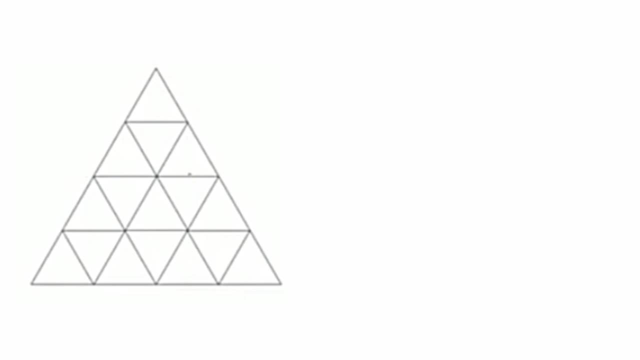 if we consider any side, we can see that there are 4 bases. So what you need to do is just write the bases one below the other, That is, 1,, 2,, 3, 4.. After that, follow these steps. Take 1,, write it. 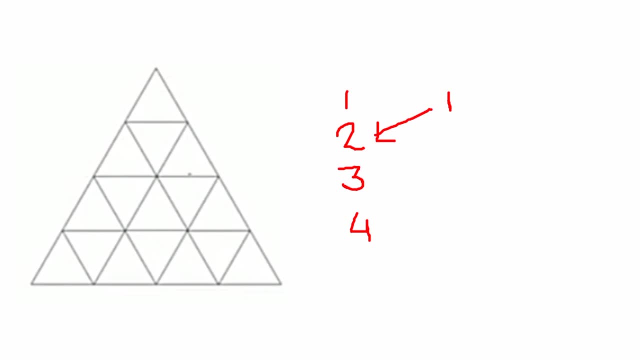 here Now. add 1 and 2. Write the answer 3 here. Add this 3 to the next number, That is 3.. 3 plus 3 is 6.. Add 6 with the next number, That is 4.. 6 plus 4 is 10.. Then add all these numbers, That is 1 plus 3 plus 6 plus. 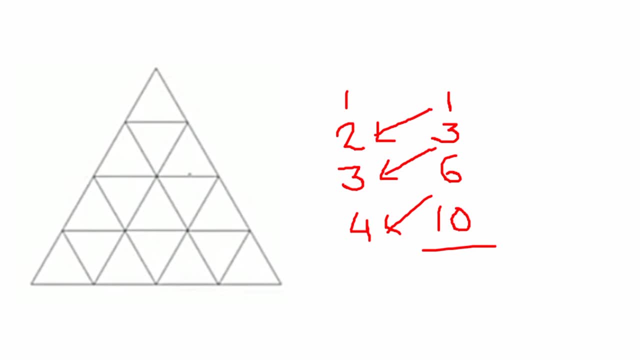 10.. 1 plus 3 is 4.. 4 plus 6 is 10.. 10 plus 10 is 20.. Then what you have to do is just look from the bottom. Leave the first number, Then add the next number. That is, 1 plus 3 plus 6 plus 10.. 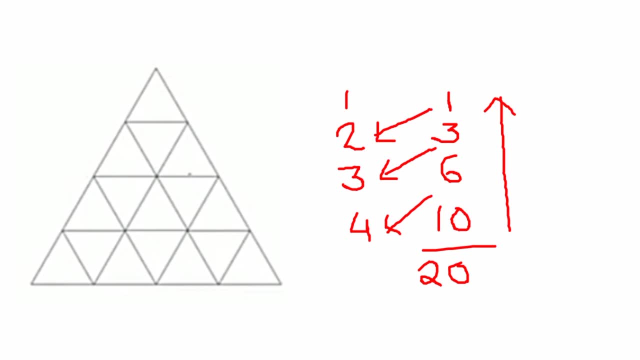 Add the alternate numbers, That is, you have to leave 10.. Add 6 plus leave the next number, Then add the next number, That is 1.. So you will get it as 20 plus 6 plus 1. That is, 27 triangles are.